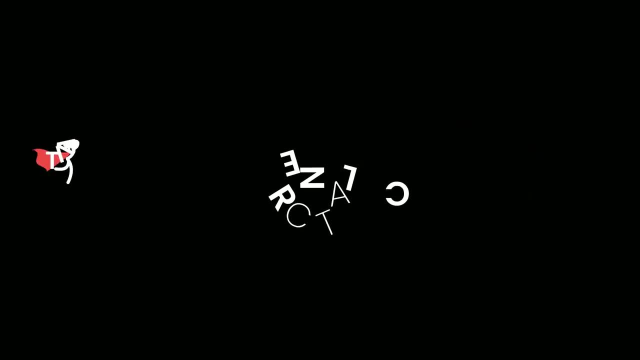 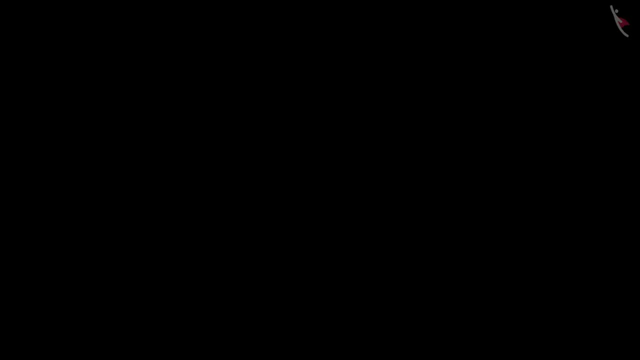 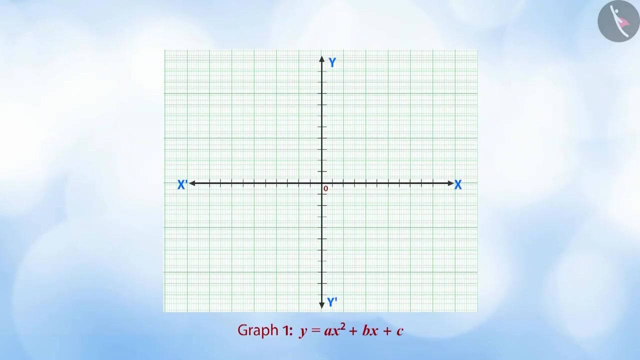 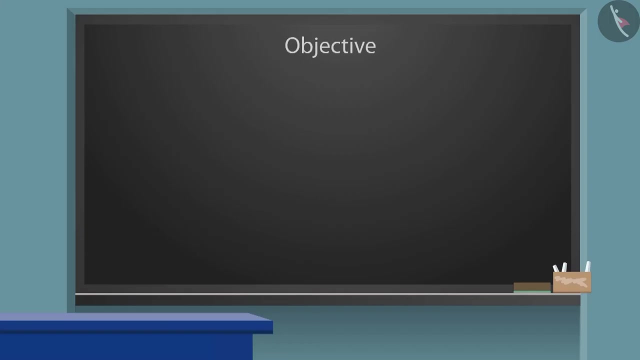 Welcome to this video. So far, we have read about the geometric meaning of the zeros of polynomial. Today we will see how the zeros and coefficients of polynomials are related to each other. In your previous class you have learned that a zero of the linear polynomial 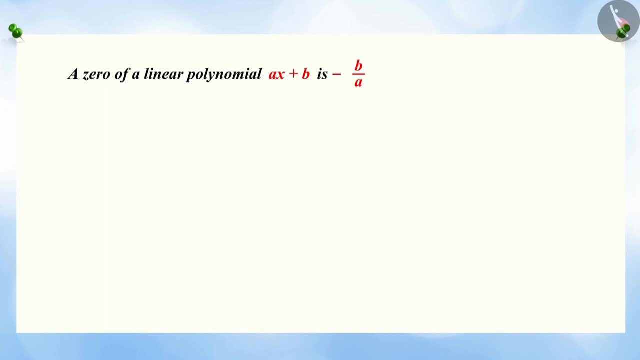 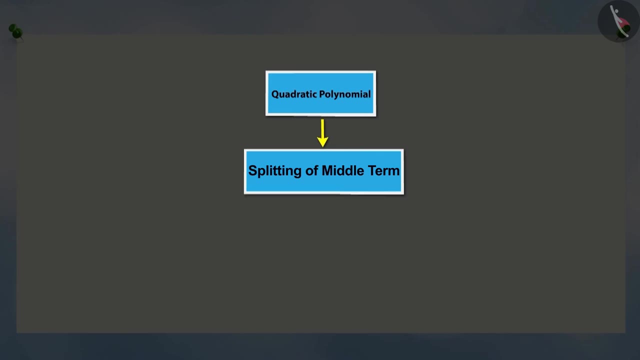 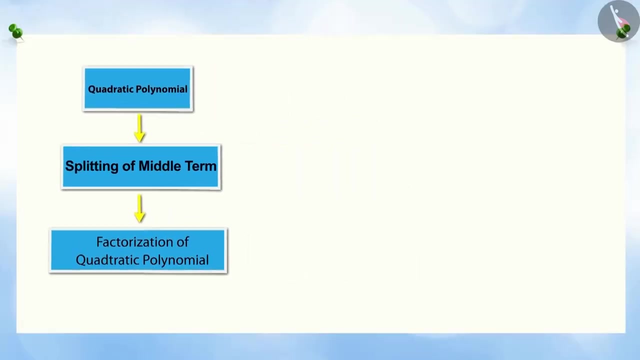 AX plus B is negative B by A. Do you know that by splitting the middle term of a quadratic polynomial, it can be factorized? For example, the polynomial is 2X square minus 12X plus 16.. The term minus 12X is written as the sum of two such terms. whose product? 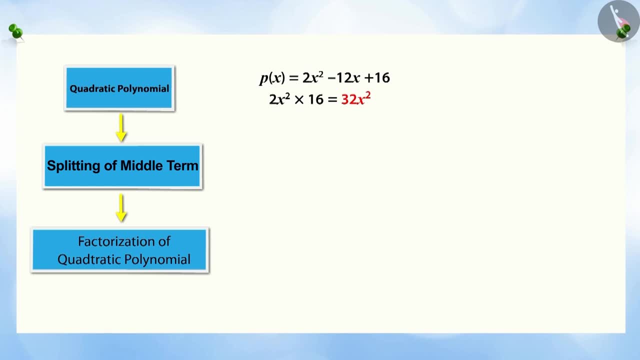 is 32X. square. On further solving, we get the factors of this polynomial. Therefore, for X minus 2 is equal to 0,, that is X is equal to 2, or X minus 4 is equal to 0,, that is X is equal to 4.. The value of 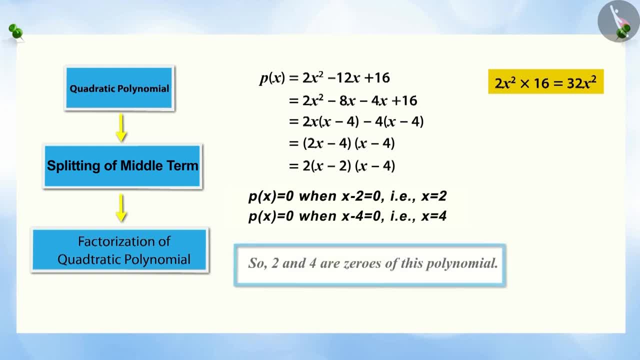 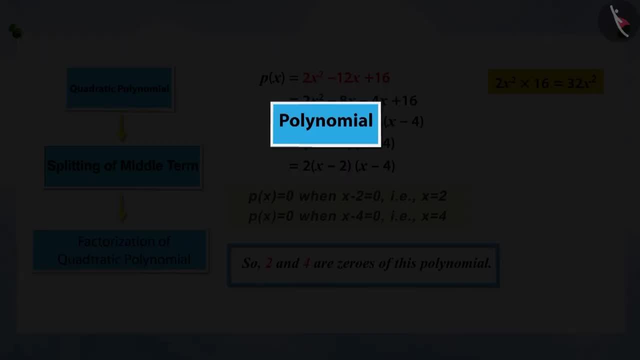 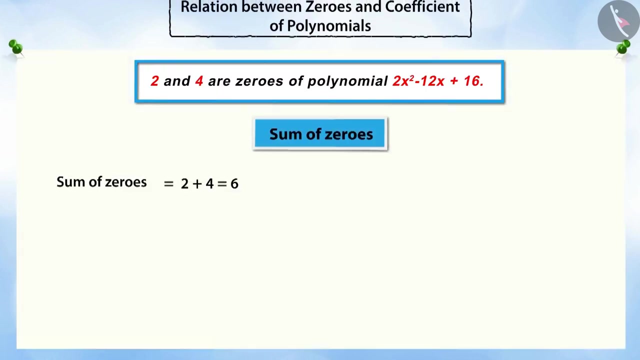 polynomial will be 0. So 2 and 4 will be the zeros of this polynomial PX. Do you know that the zeros of polynomial and coefficient are related to each other? Let's see how. If we add zeros, you will see that the sum of the zeros is equal to the negative ratio.